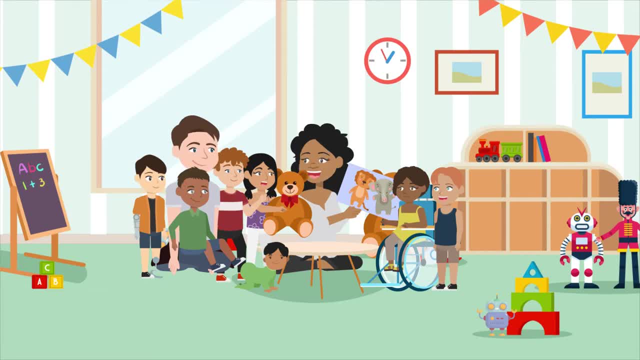 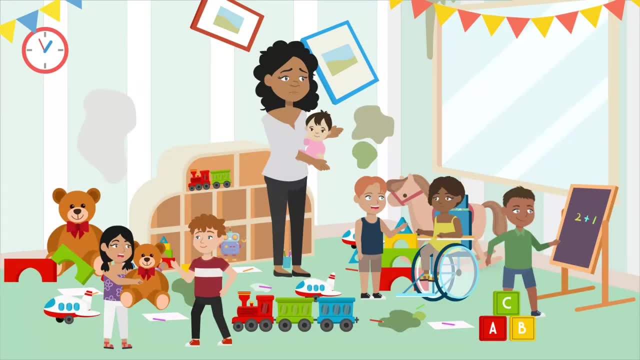 And to be able to stay close to children who may need additional support. Face into the room. when sitting at a table with children, for example, Make sure that there are always clear paths to where children are and safety concerns are addressed, so you can react quickly when necessary. 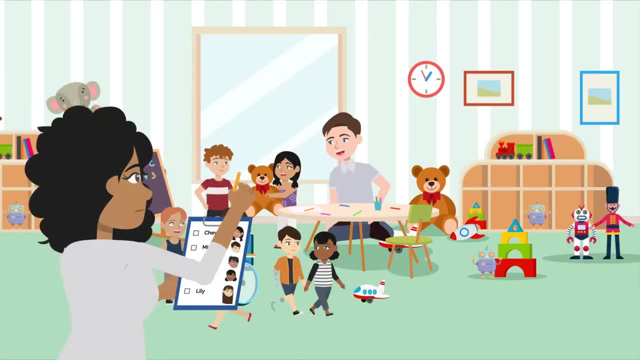 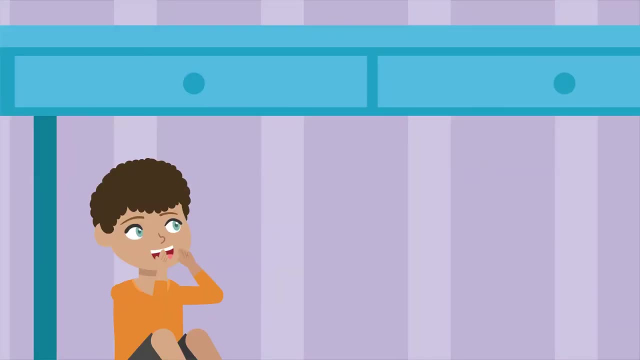 Keep an eye on the children at all times by scanning the room and regularly counting kids to make sure no one is missing and checking the sign-in sheet to ensure the count is accurate. A face-to-name check is always a good idea. If you don't see one of the children, first check all the areas in the vicinity where 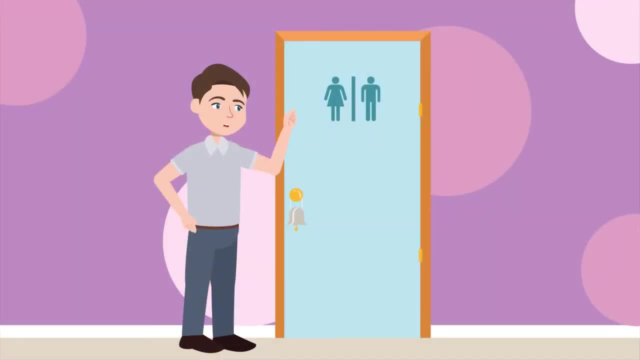 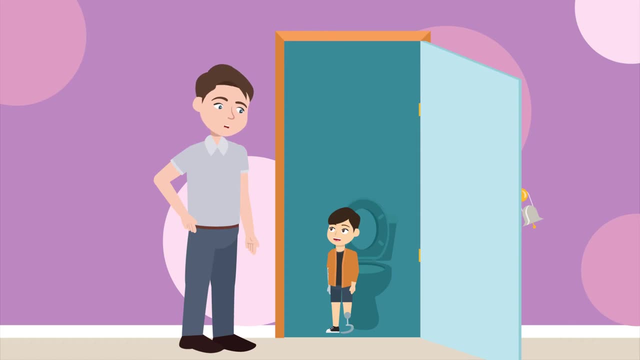 kids might hide. If a child doesn't return quickly from a bathroom trip, make sure you check on them. Consider leaving a bell or some other type of noisemaker on the door to alert you when someone is entering or leaving. For a two-year-old, it seems there's no greater thrill than to escape. 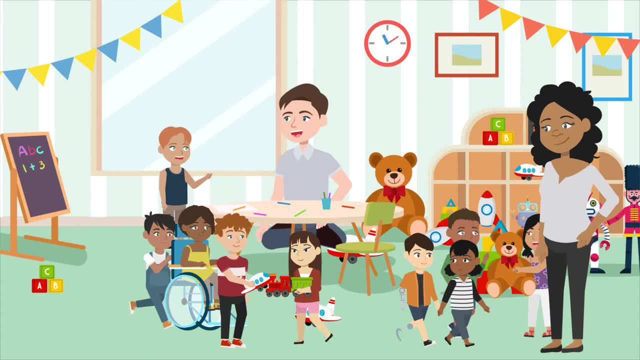 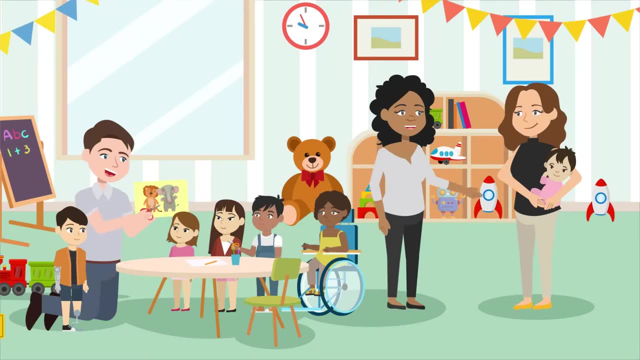 It's hard enough to keep a count of a fixed number on children all day, but when that number fluctuates it can be twice as difficult. Make sure you have a process in place to allow for any children who might arrive late or leave early, so that your group count is always updated accordingly. 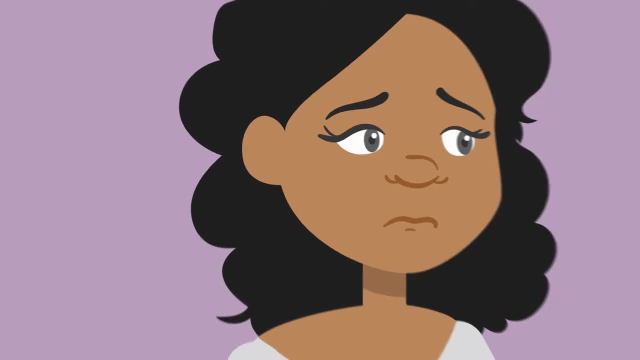 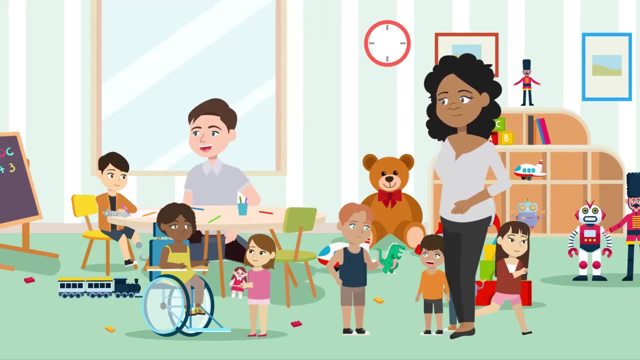 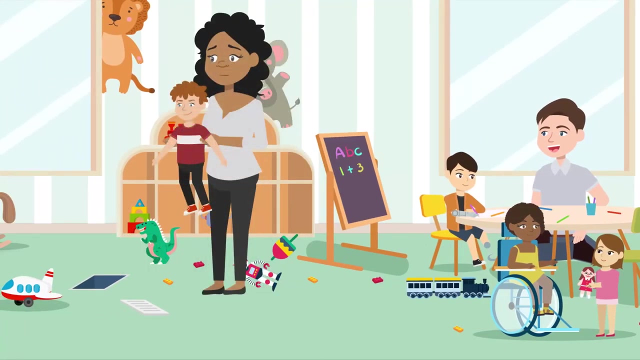 Your ears will tell you a world of information if you pay attention to them. We all subconsciously recognize when the normal soundscape around us changes, but you need to be more attuned to your surrounding sounds when caring for children. Specific sounds or the absence of sounds may signify a reason for concern. 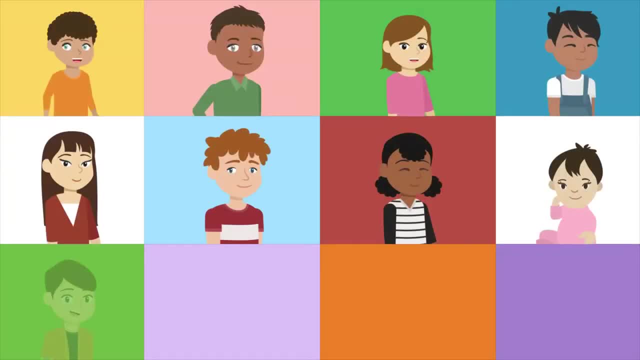 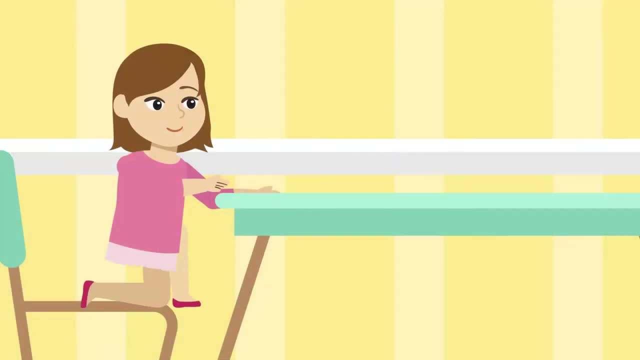 Use your knowledge of each child's individual development and abilities to anticipate what a child may do. You see them on a daily basis. You know their quirks. Does one of your kids climb, Or several? Does one like to burrow under blankets? 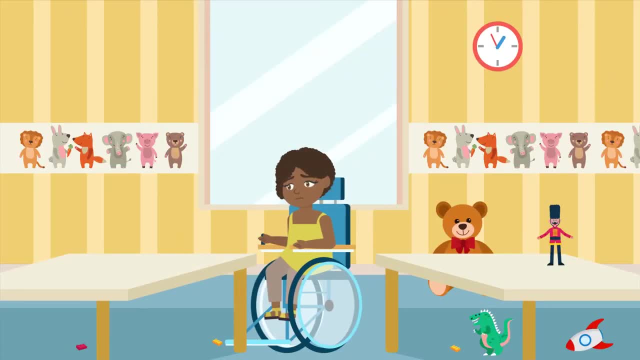 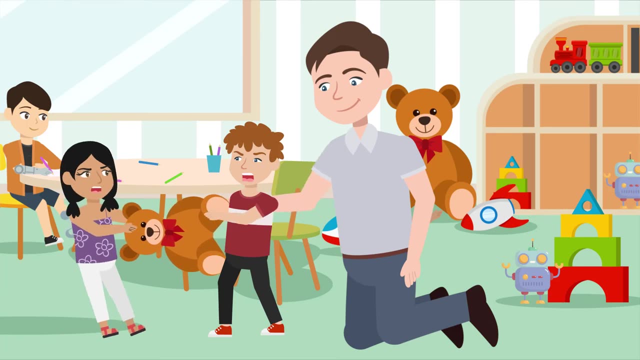 Or into small private places? Are there known circumstances where issues are more likely to occur? The best way to prevent issues is to guide them and redirect them when necessary before the issue arises. This only happens with regular engagement. If you have any questions, please let us know in the comments below. 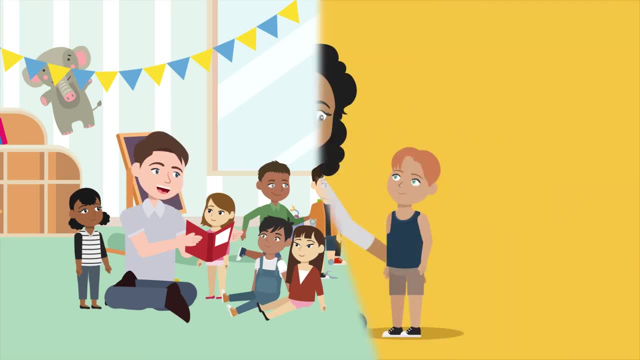 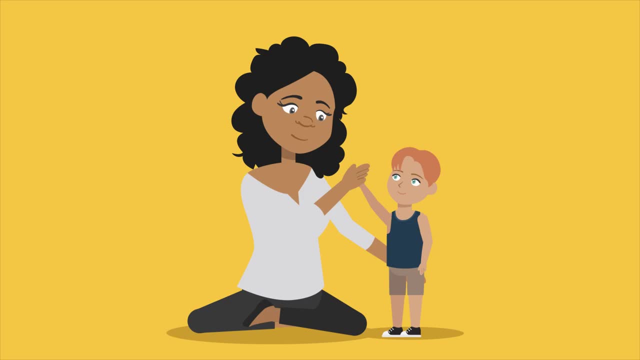 And the best engagement is joining them in play. The more you engage with them and provide active supervision, the more you can prevent issues from arising and improve children's safety. Children are truly our most precious resource and it's only right that we take the utmost. 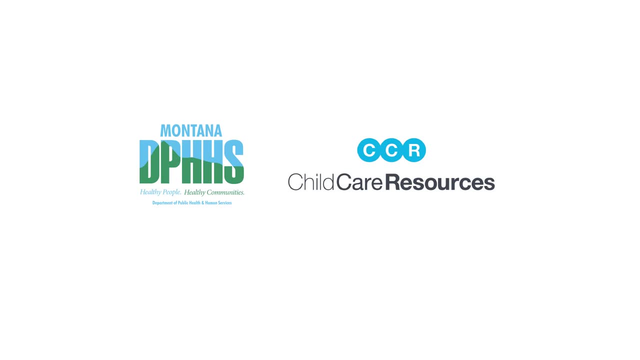 precautions in ensuring their safety while they are in our care.